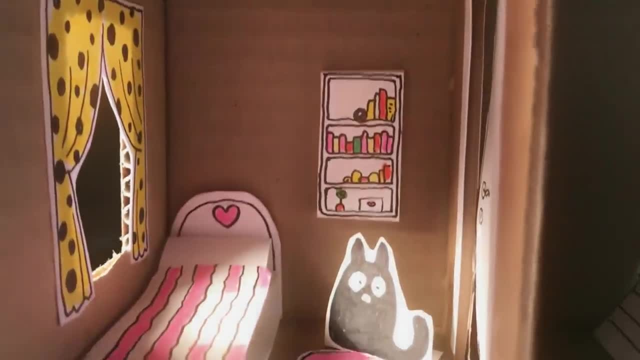 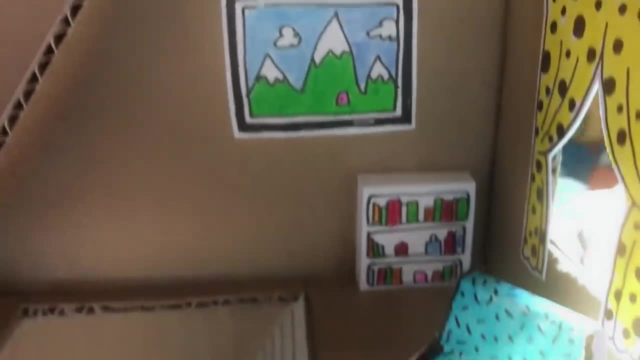 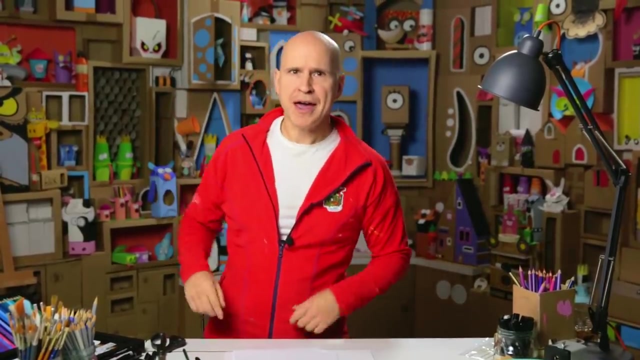 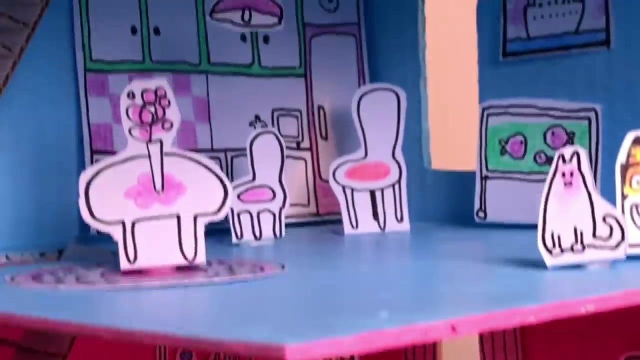 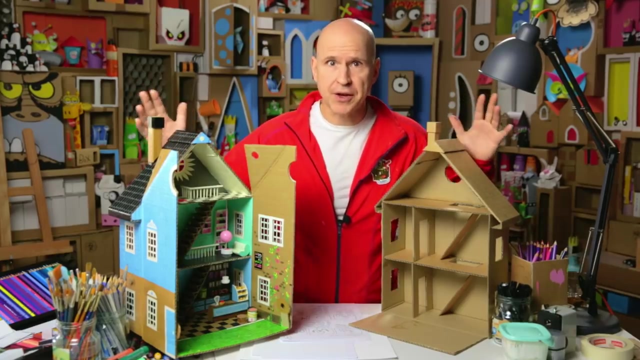 Why? everybody good to see you. Have you seen this pink dollhouse yet? In this video I promised to show you how to draw the characters in the house and the furniture. Here I have two more houses that I have made in earlier videos. Check them out if you haven't seen them. 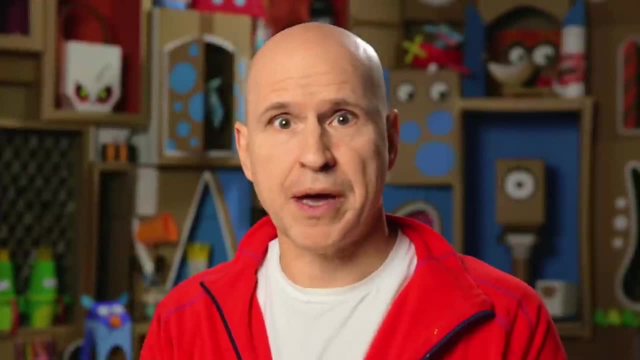 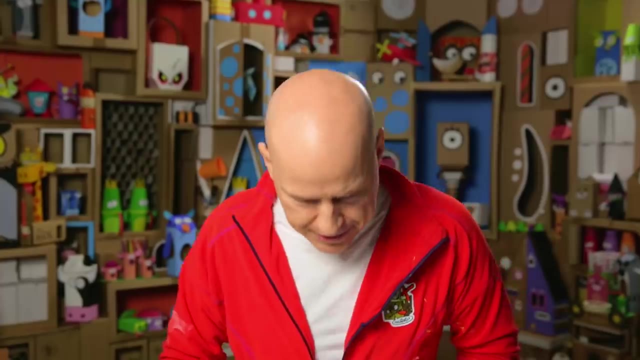 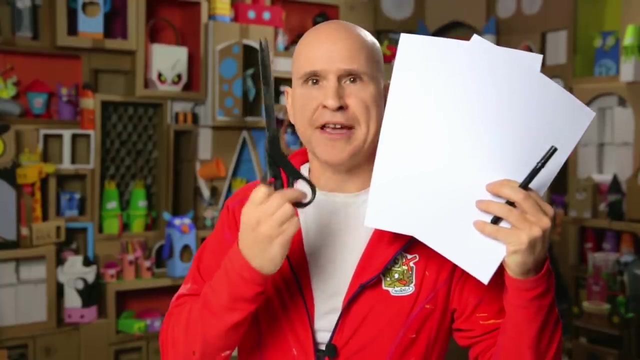 They're awesome. Now I'm going to show you how to make people pets and furniture for any house that you build, And all you need pretty much to make it is some thick white paper, a marker and a pair of scissors. Well, it doesn't have. 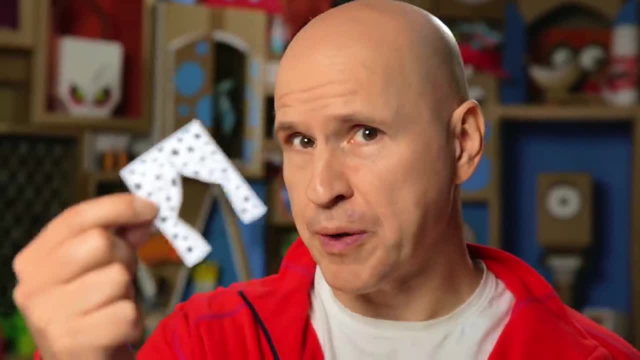 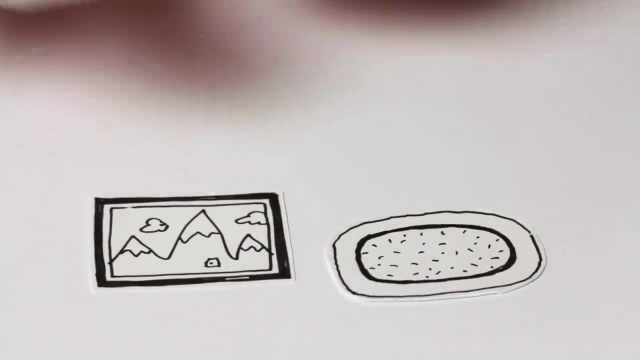 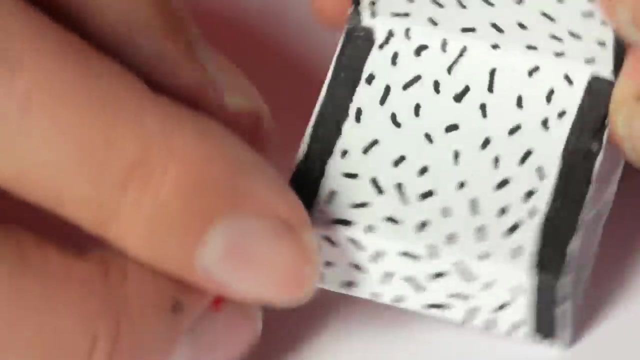 to be this big. All we need is to draw what we want and cut it out. We can draw a flat things like this carpet or this painting, or we can fold the drawing at the end so that it can stand up, Or fold the paper and make the furniture totally 3D. Let's take a dining. 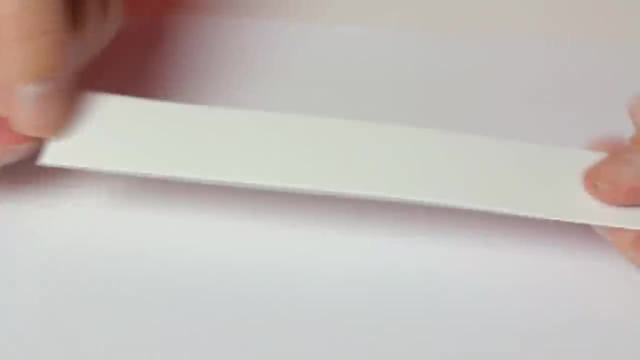 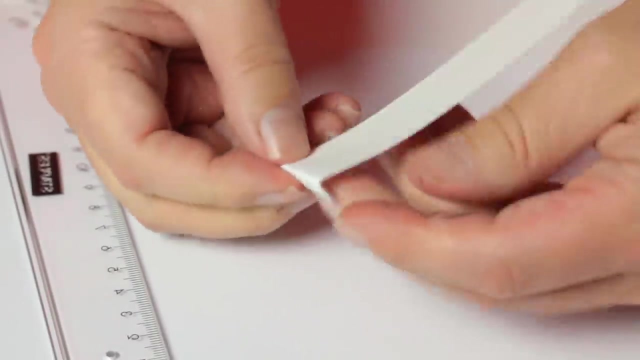 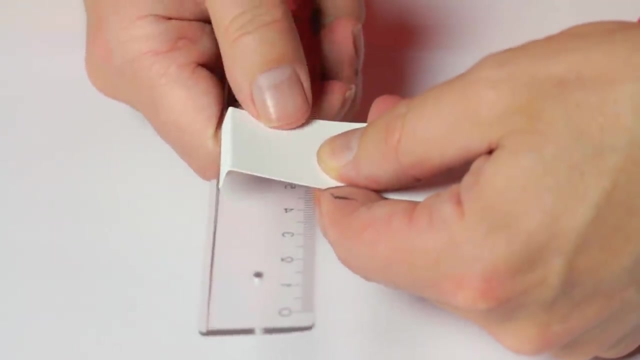 table. We will certainly need that in our house. Here I have a strip of quite thick paper. First I make a little fold. This fold will stabilize the table on the floor. Then the height of the legs will be about this high, like that. Then I have to decide how. 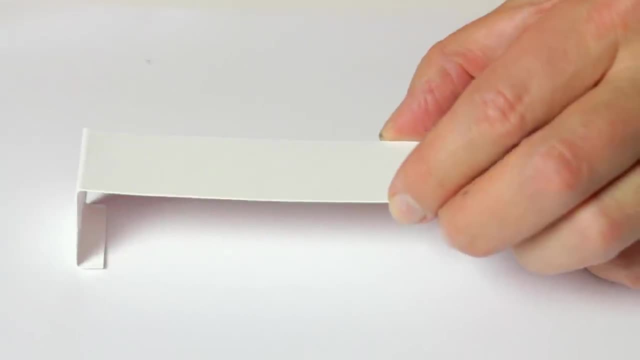 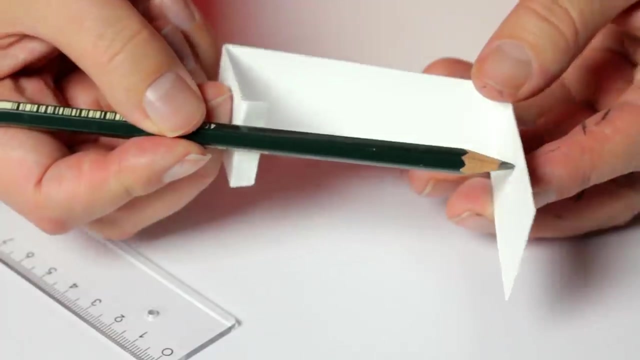 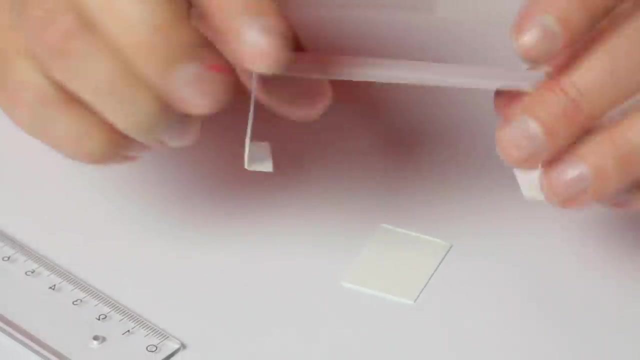 long is the table going to be? Maybe about this long? Make a fold here, Then I have to match the height of the legs there. Fold here, Then I make a cut so it's equal on both sides. A decent dining table. 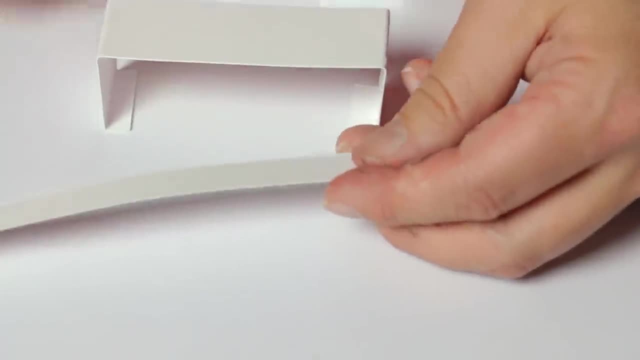 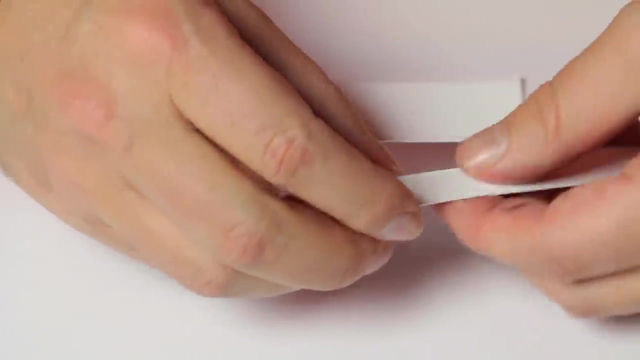 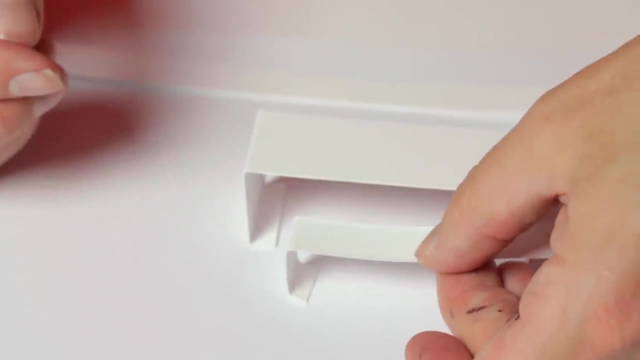 Now let's make some chairs. I got some thinner strips of paper. Let's make a little fold to stabilize the chair, Just like that. How high should the seat be? Maybe about. oh yeah, I think that's a very decent height for the chair. The seat should be about that wide. 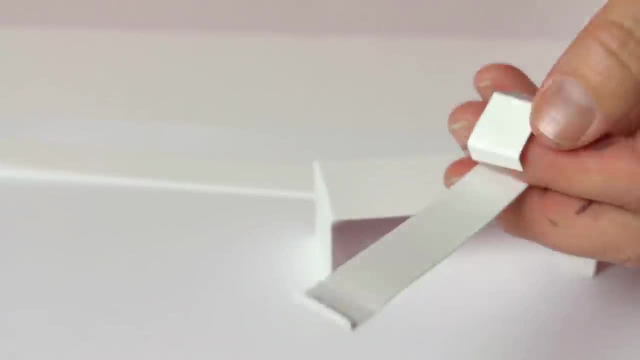 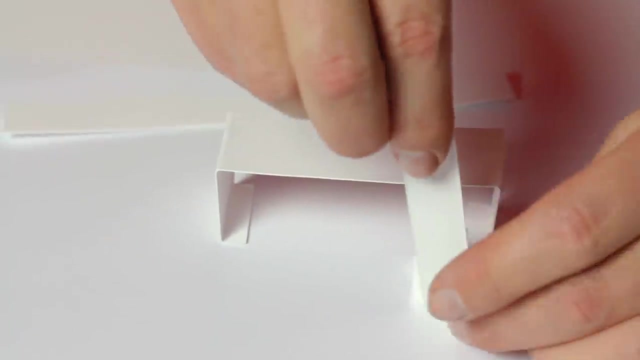 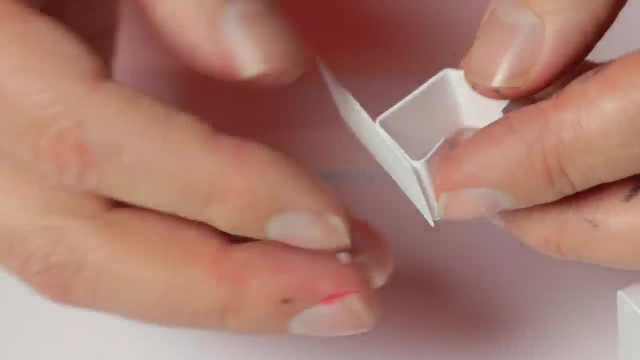 Making sure the legs are the same height. Then I can snip this off. Yay, Nice. So now I can make the back of the chair The same strip of paper That high. A little bit of glue on the back there, Put this together. Nice one, Nice one, Yeah, All we need to do. 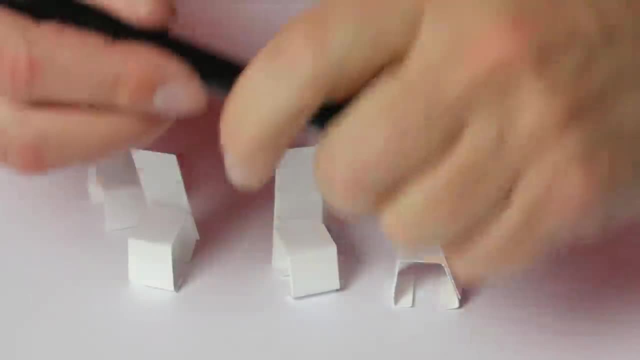 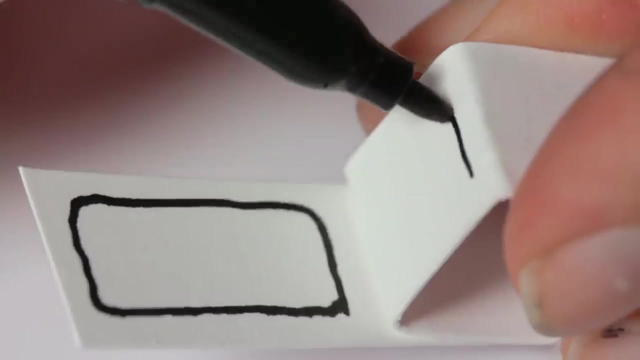 now is to make a few more of these There. Four chairs Now. maybe we should decorate them a bit too On the back, Maybe a little cushion here And a cushion on the seat to make it softer to sit on. Yeah, nice. So now I can make the back of the chair The same strip of paper That high. 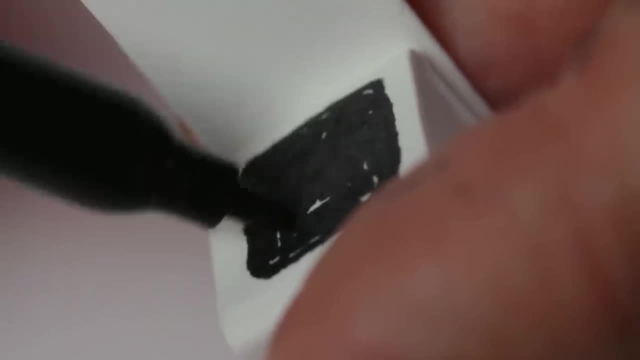 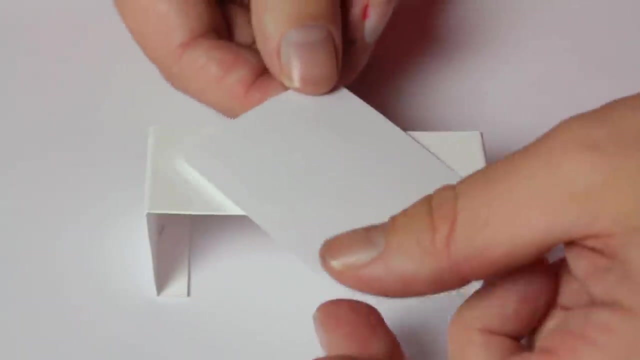 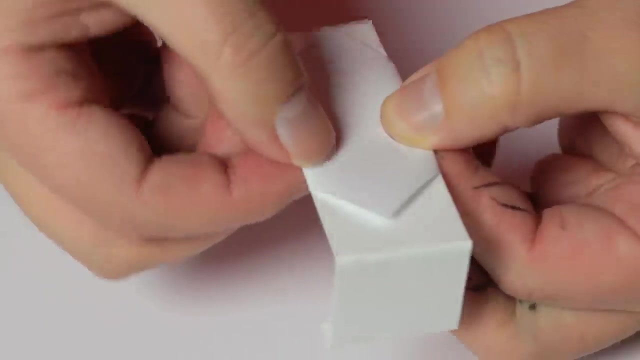 Maybe a little cushion here And a cushion on the seat to make it softer to sit on. Maybe color this in. Now, what do we put on the table? How about a little tablecloth? Yeah, I've cut a little square, So let's see now if we fold it here And here It should. 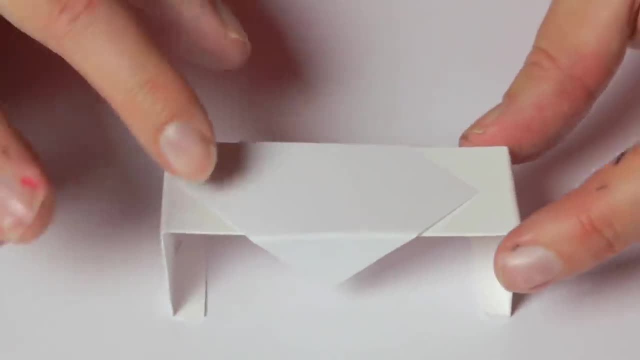 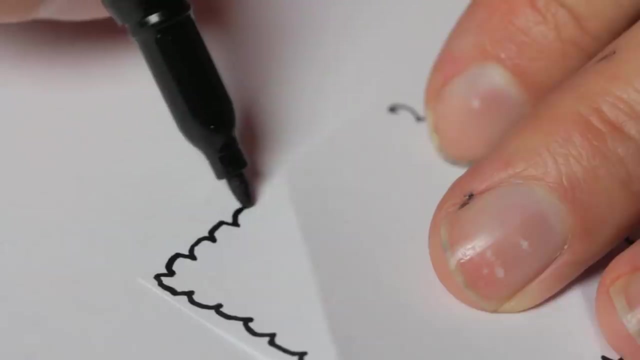 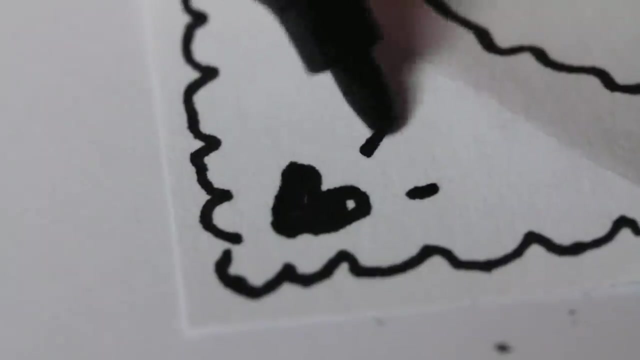 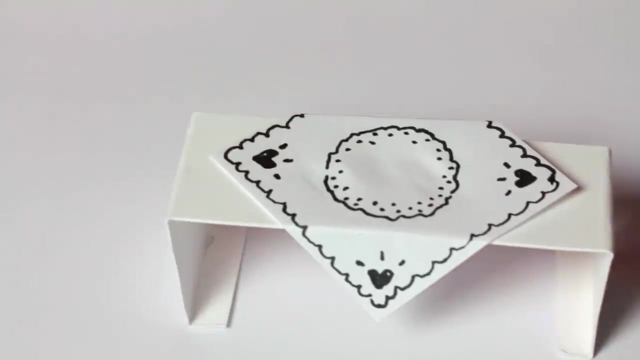 fit just beautifully. So oh nice, But we need to decorate it a bit. So what shall we draw? Let's draw a little tablecloth pattern, A little bit of glue, And on it goes Gorgeous. Check some of the other furnitures that I. 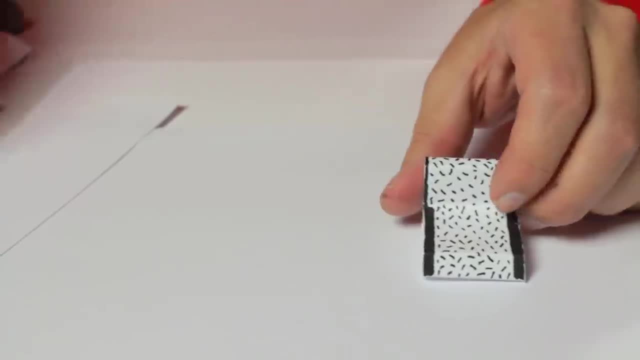 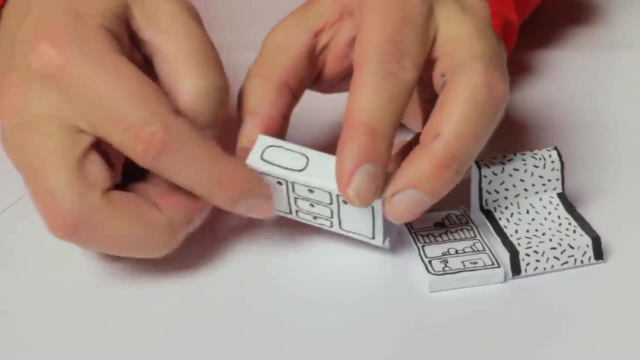 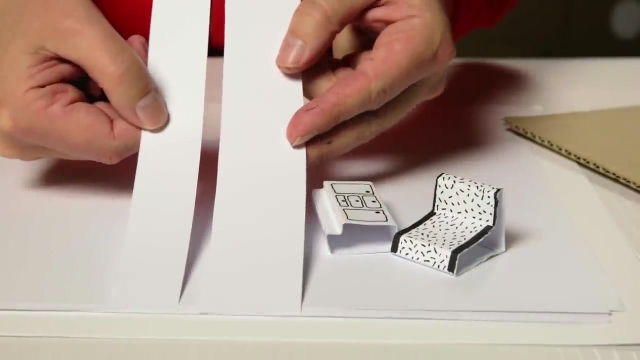 made A cozy little sofa. Here is a neat little bookshelf. Have about a piece of bathroom furniture with drawers and a sink on top All these things. It's been a long time since I've done this. I think it's very easy. I just use different types of strips of paper. 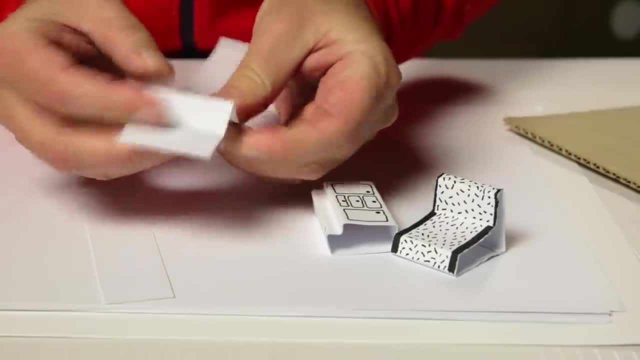 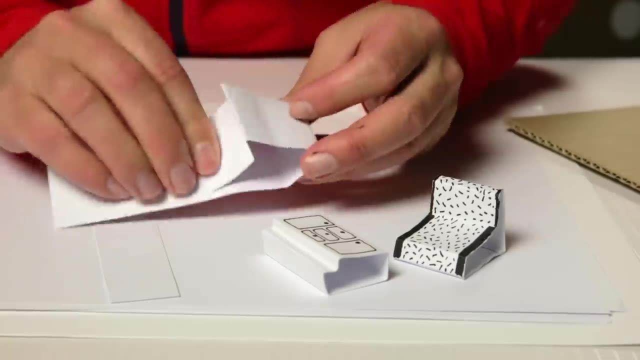 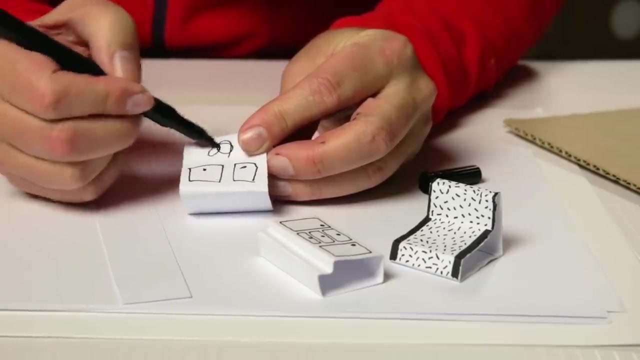 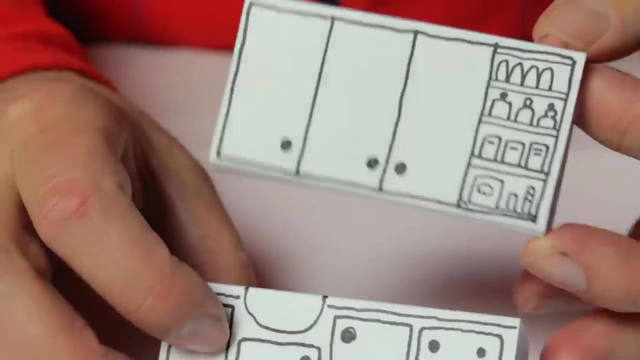 I make folds anywhere I like, Glue them together at the end, However shape I like to have, And then I draw on the features with a marker anyhow I wish. Check out the kitchen gear, Look at that- The big cupboards- and stuff up here, And then 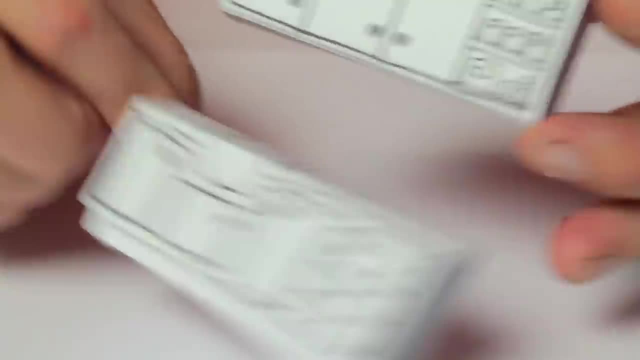 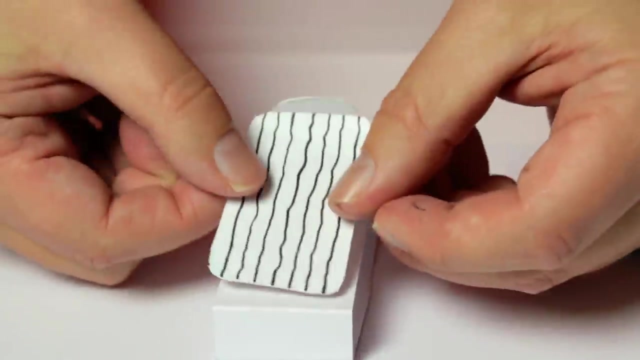 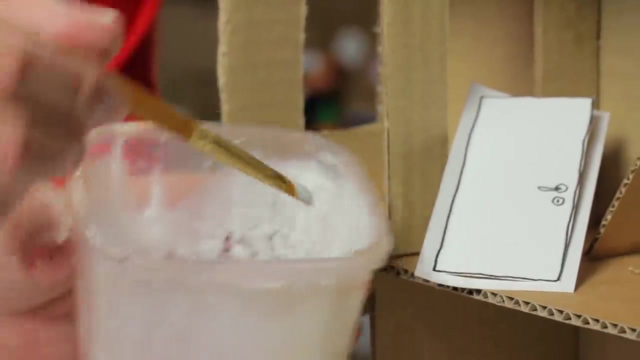 here is the drawers and the sink, The two sinks. Oh, look at this Bed Like that, Like that, With a nice pillow And a cozy bed sheet. Oh, nice. Let's start with the doors and the door frames. I dip brush in glue. Put it on the sides here. 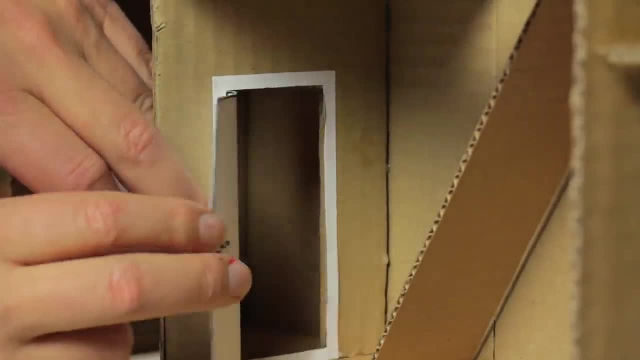 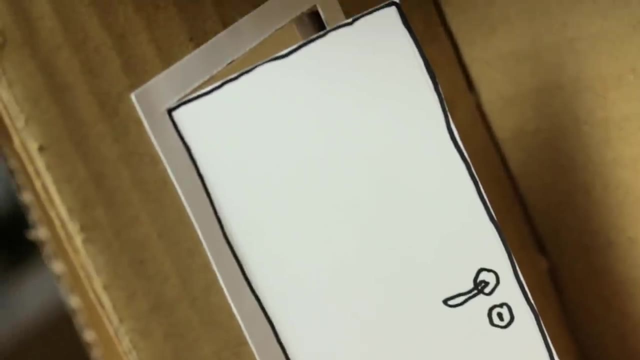 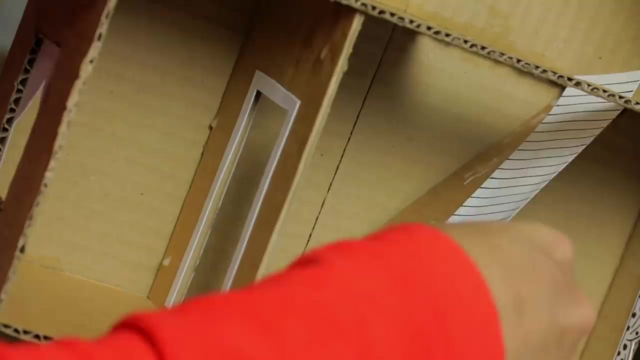 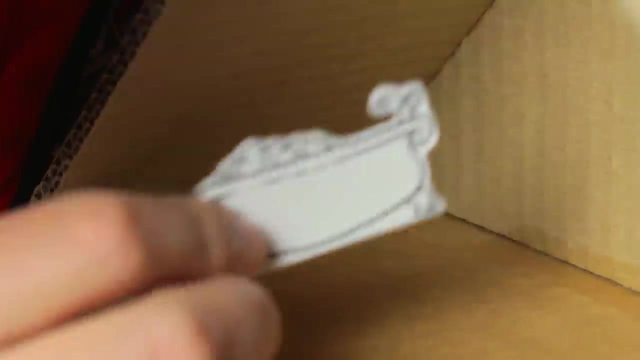 Stick it on Now it can open and close. And the other one downstairs. Curtains in the windows Window frame for the bathroom Staircase. Look how simple I drew that. Let's start the interior decoration. We start with the upstairs bathroom first. 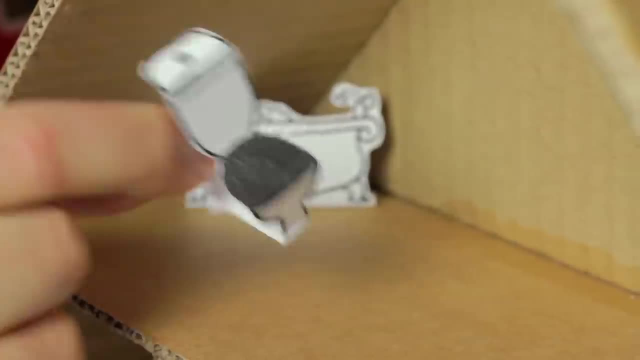 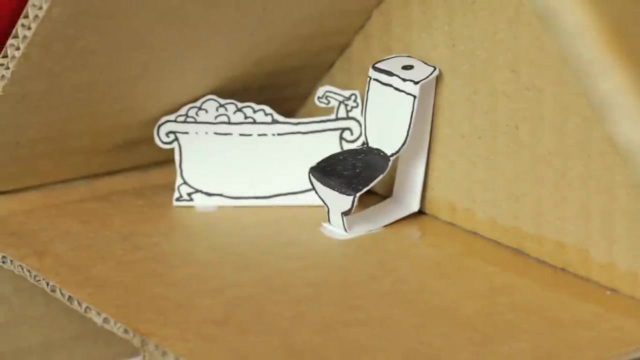 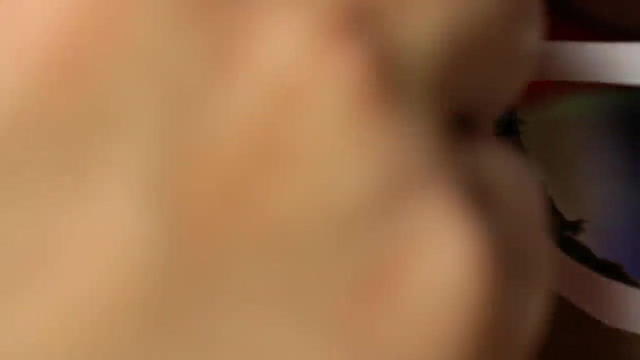 And here is the bathtub, Then the toilet. Check out the toilet. Isn't that neat. Okay, It goes here right next to the bathtub. Then the bathroom drawers with the sink on top And a little mirror on top of the sink. 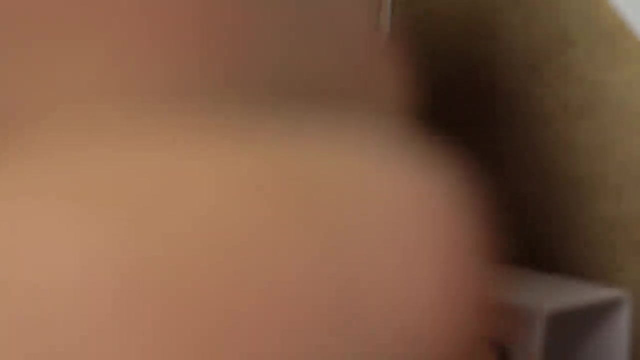 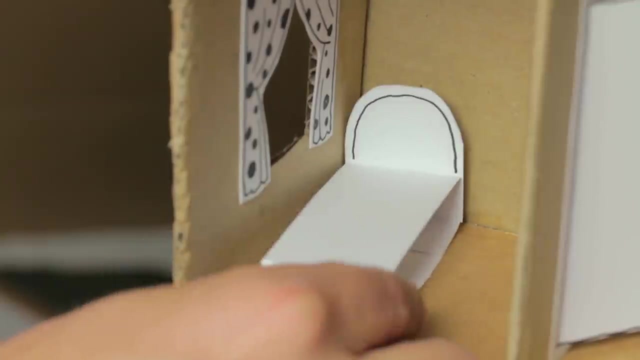 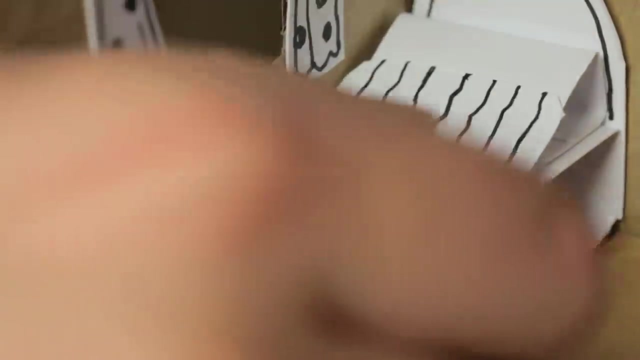 Bathroom carpet, Nice and soft, And we mustn't forget the tap. Can you see it Right over there by the sink? Then we move down to the bedroom with the bed, of course, Not to forget the pillow And the soft and nice cozy duvet on top. 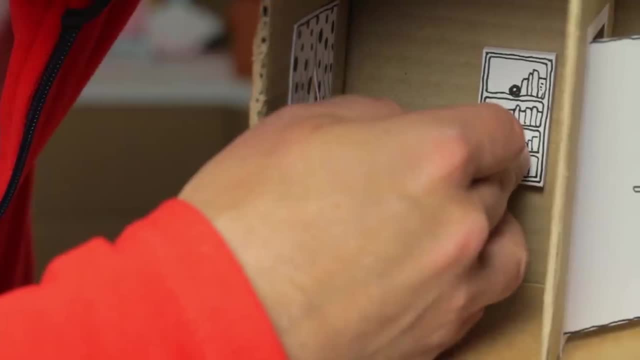 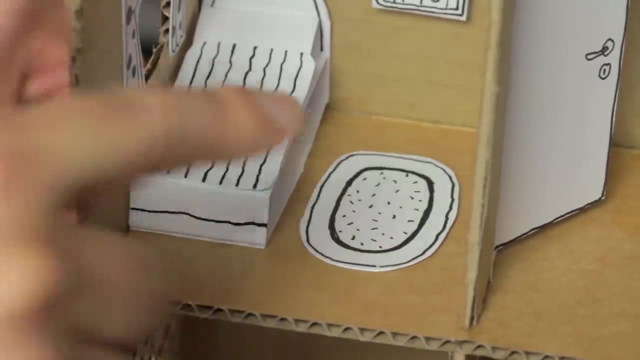 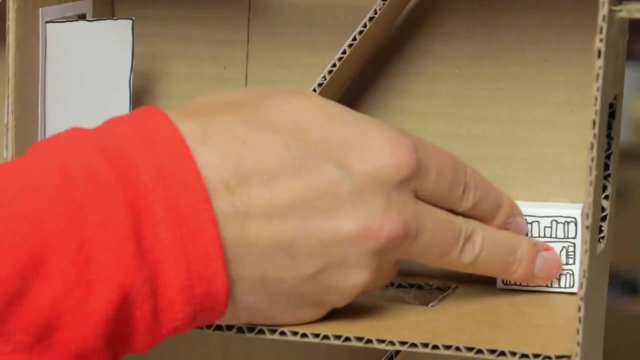 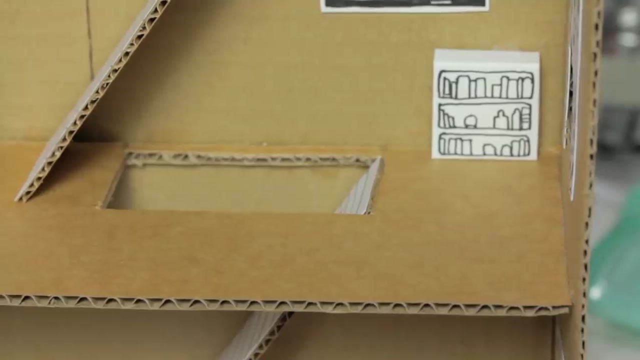 The bedroom will need a little bookshelf- We'll mount it on the wall- And a little soft carpet on the floor right by the bed And a generous Japanese lamp in the ceiling Bookshelf in the living room, And above the bookshelf, a little oil painting of the landscape. 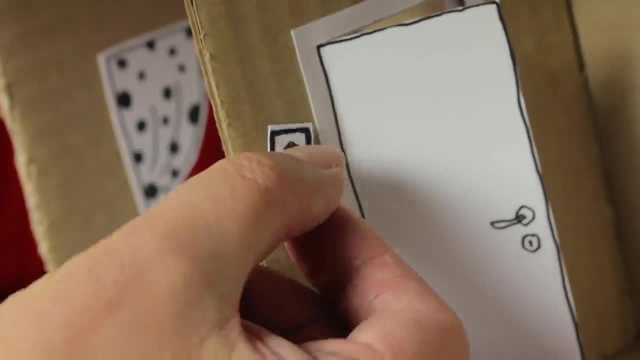 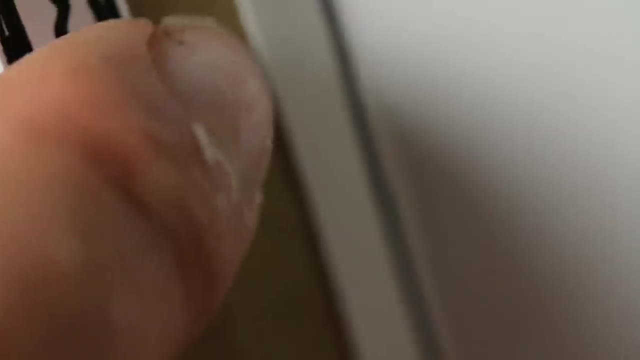 Sofa Carpet on the floor, A picture on this very small wall. It's a portrait of old granddad when he was young. There's a picture of an old man with a bit of a brain And another picture on the granddad. 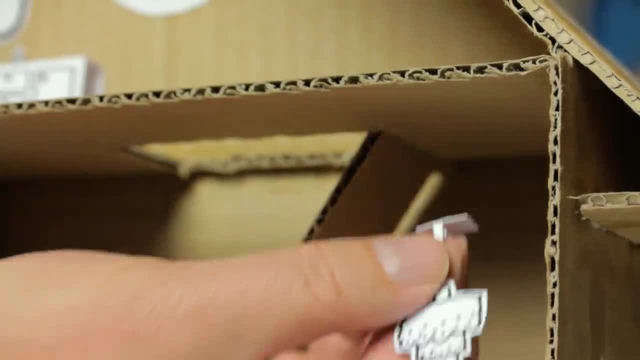 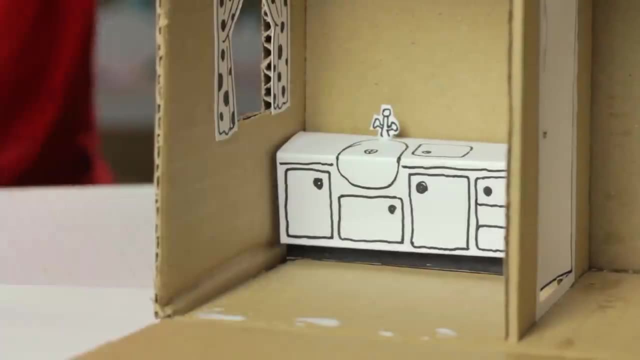 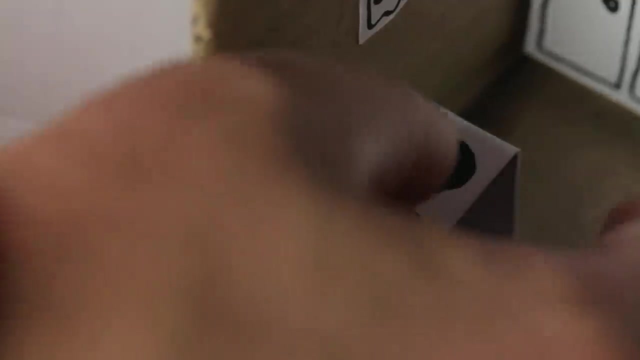 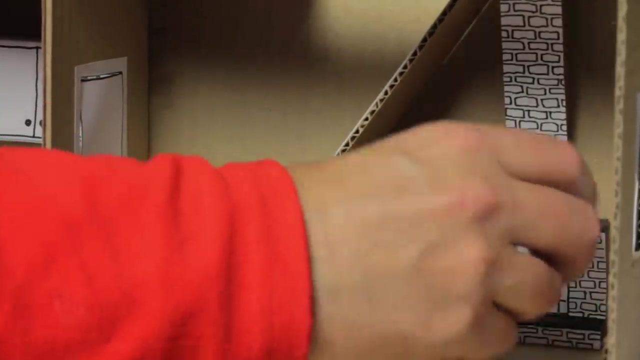 I don't know what that is all about. And a gorgeous chandelier in the ceiling. Then we move down into the kitchen. First the kitchen sink, Then the cupboards above the sink And finally a cooking stove, Fireplace, yeah, right in the dining room area here in the back. oh beautiful, look at that. so nice and cozy. 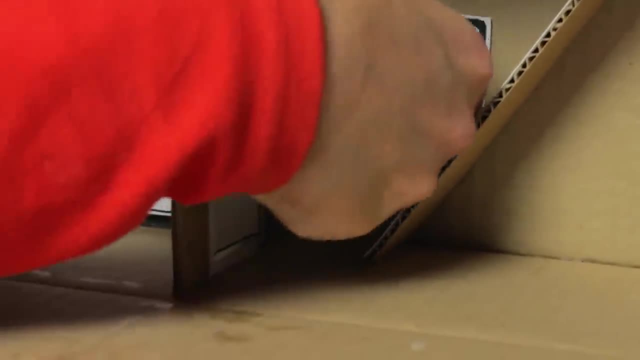 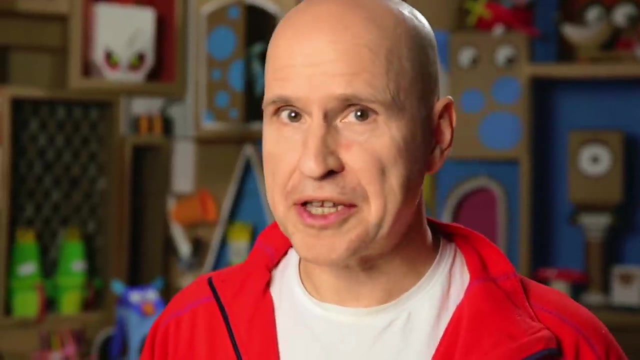 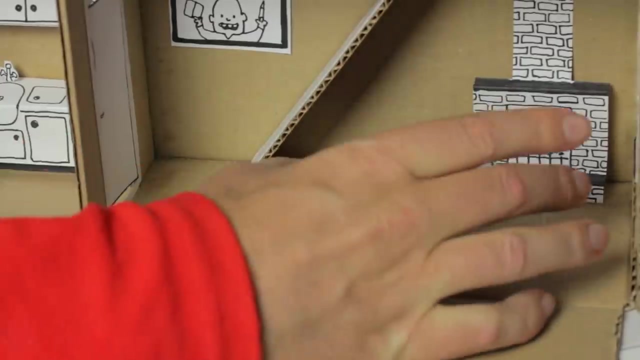 big size flat screen showing box yourself. yeah, what else goes up on the wall there? and let's add in the dining table and the chairs that we made earlier. i think it should go right here, quite close to the fireplace, but not too close. and then the chairs there over here, beautiful. 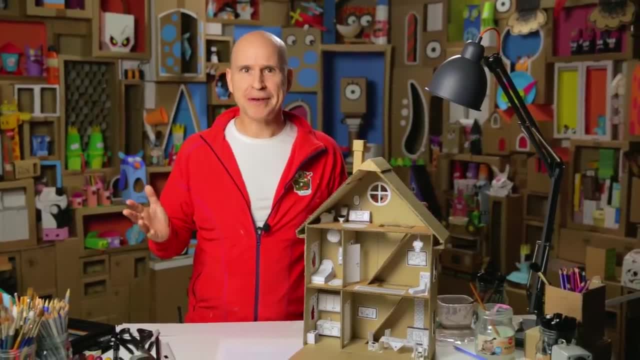 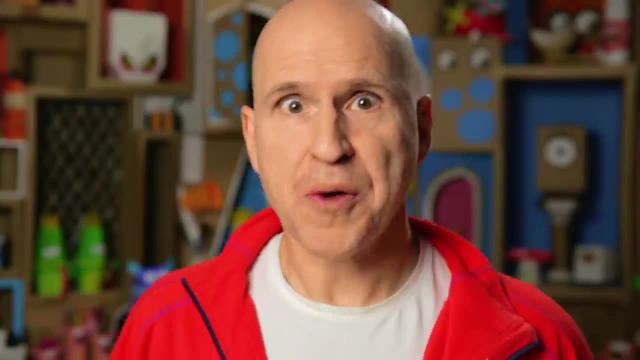 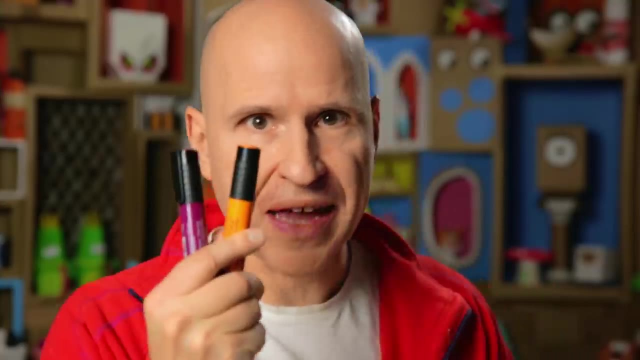 now you may wonder why everything is in black and white. well, it's all up to the style that you choose. having an all black and white house is really cool, but also when everything is in black and white and cardboard brown, any color that you put into it will stand out and look good. let's try. 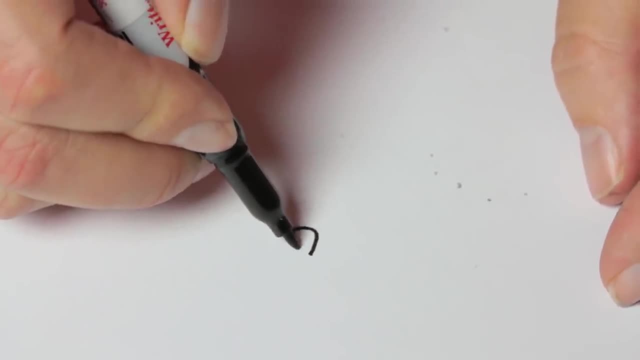 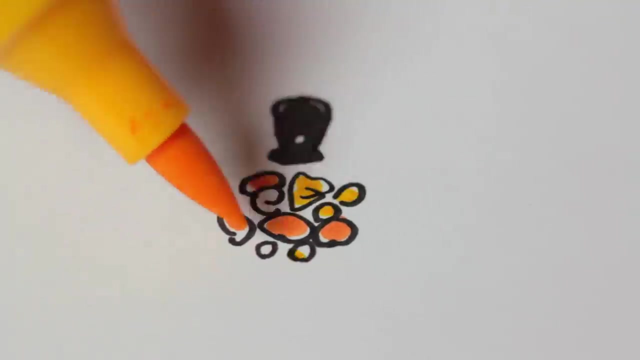 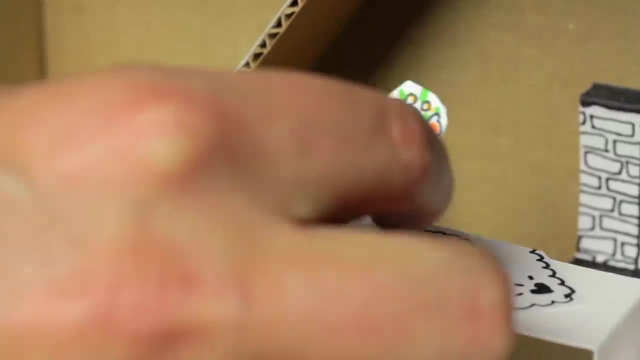 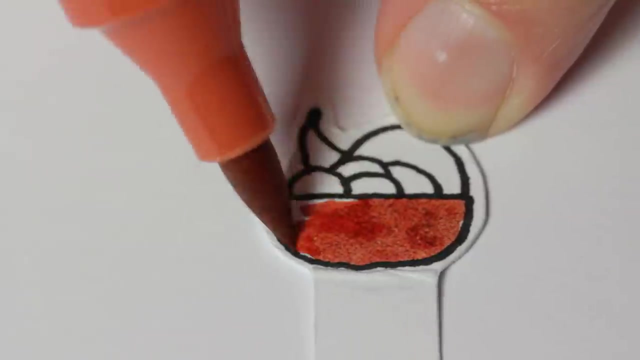 a vase of flowers. so here is the vase, color it black, then the flowers, and then we color them in, cut it out, then we fold a little gluing lug. let's put it here on the table, oh gorgeous. or have about a bowl of fruit right on the kitchen table and a bit of color. 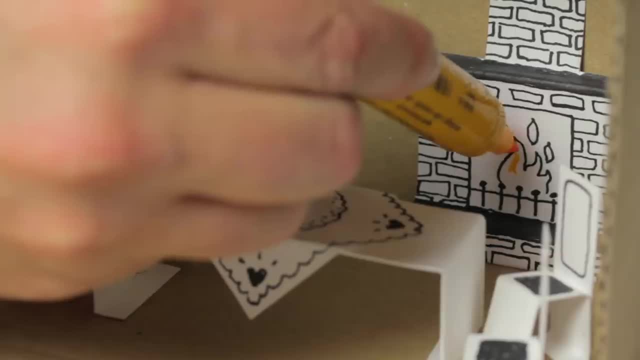 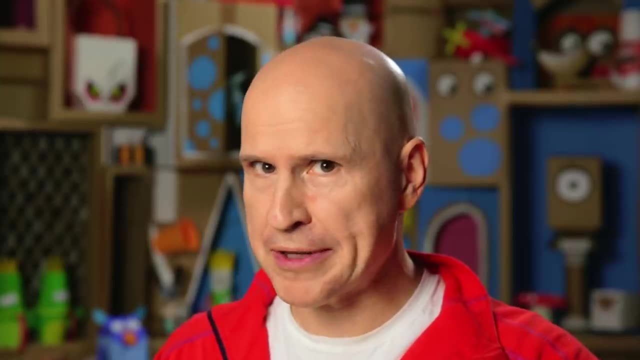 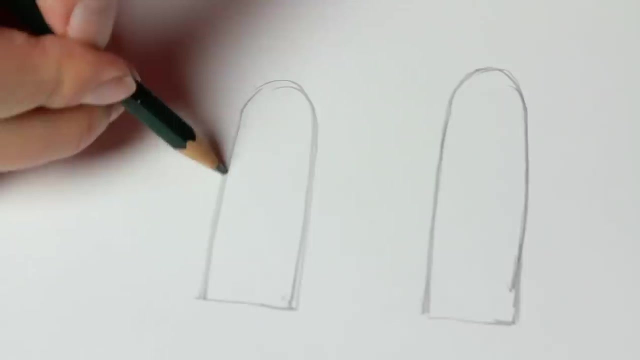 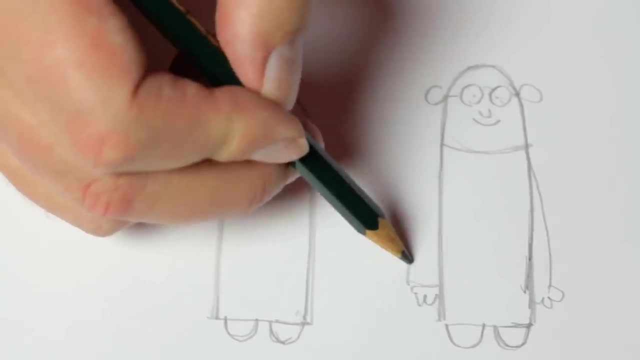 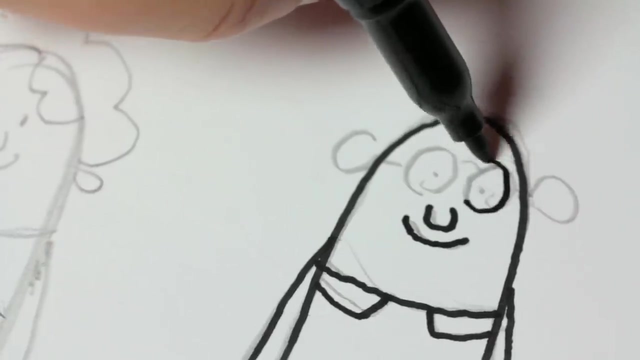 on the floor, fireplace. what else do we need? people, of course. here's mom and dad. i start with sketching the basic shape. so there is that. there is mom, some shoes now for the face. yep, here is that little hands there and mom. then i ink them in, erasing the pencil marks and color in. 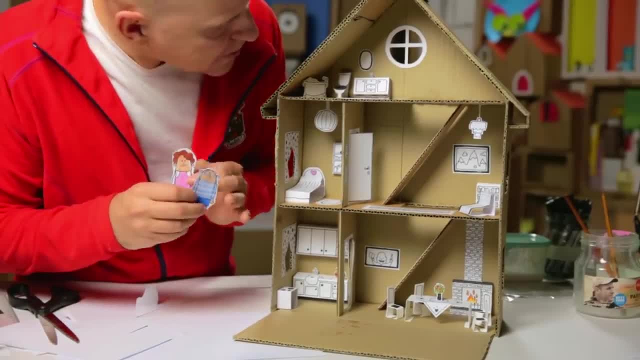 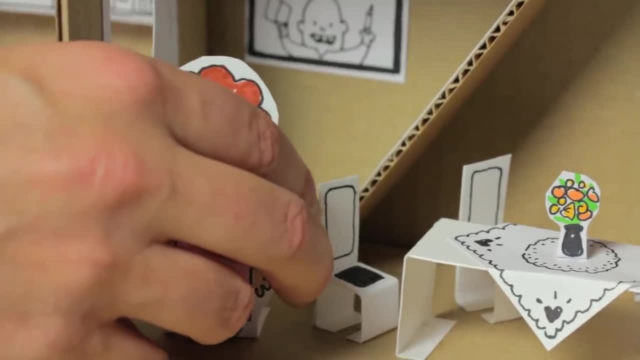 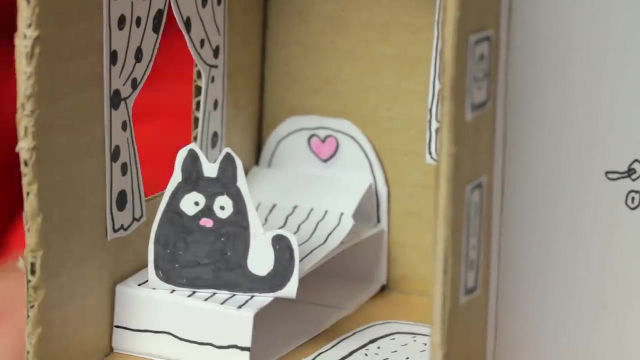 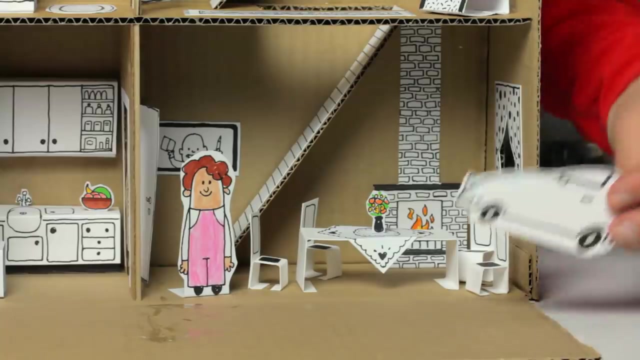 now, where shall i put them? how about, maybe that up here in the bathroom? mom can be down here in the dining room. and how about the cat? ha, yeah, sitting on the bed now. how about the kid? now you make up the kid yourself. it could be you. finally, we parked the.